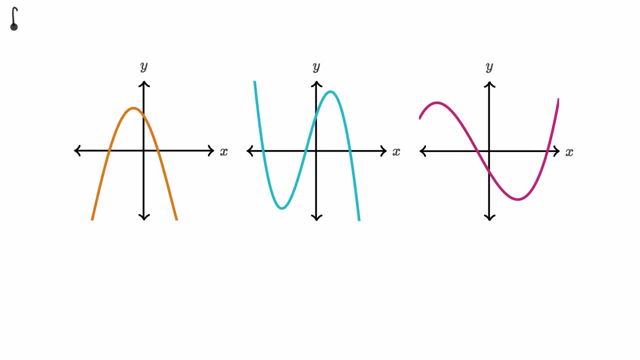 We have the graphs of three functions here, and what we know is that one of them is the function f, another is the first derivative of f and then the third is the second derivative of f, and our goal is to figure out which function is which. 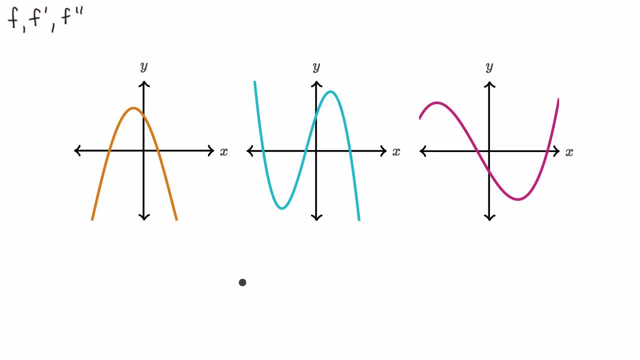 which one is f, which is the first derivative and which is the second. Like always, pause this video and see if you can work through it on your own before we do it together. All right, now, let's do this together, and the way I'm going to tackle it. 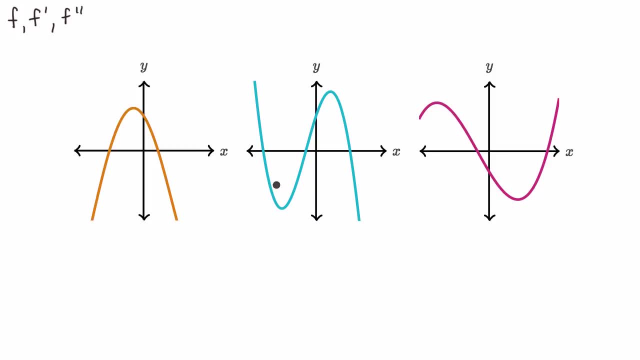 is. I'm gonna try to sketch what we can about the derivatives of each of these graphs or each of the functions represented by these graphs. So in this first graph here, in this orange color, we can see that the slope is quite positive here. 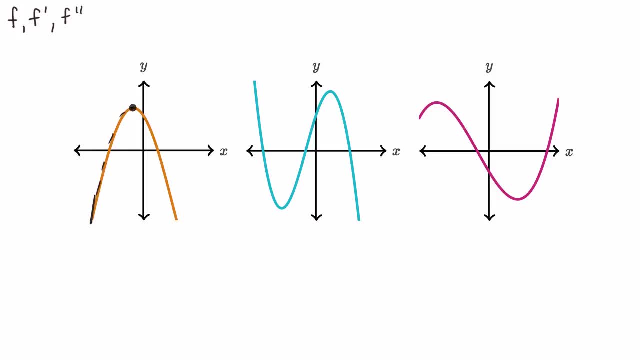 but then it becomes less and less and less positive, up until this point where the slope is going to be zero, and then it becomes more and more and more and more negative. So the derivative of this curve right over here, or the function represented by this curve, 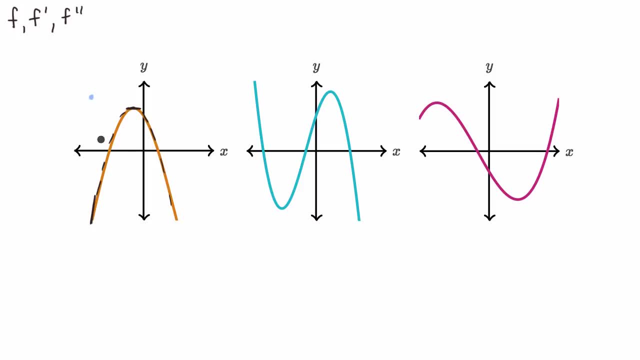 it's gonna start off reasonably positive. right over there At this point the derivative is gonna cross zero, because our derivative is zero there- slope of the tangent line and then it's gonna get more and more negative, or at least over the interval that we see. 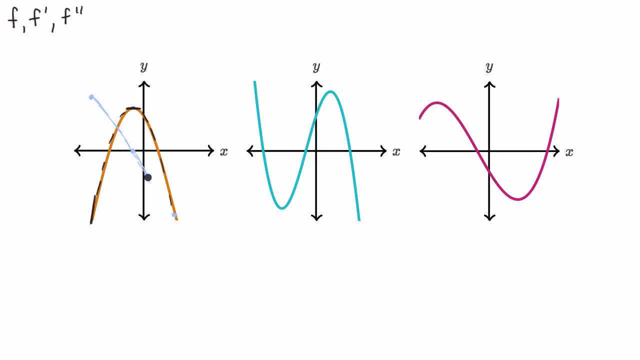 So it might look- I don't know- something like this. I don't know if it's a line or not, It might be some type of a curve, but it would definitely have a trend, something like that. Now we can immediately tell that this blue graph. 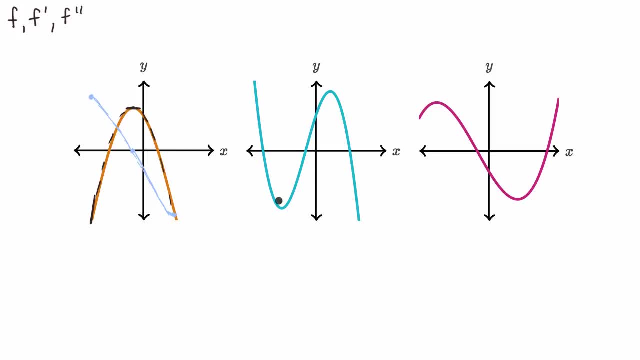 is not the derivative of this orange graph. Its trend is opposite. Over that interval it's going from being negative to positive as opposed to going from positive to negative. So we can rule out the blue graph as being the derivative of the orange graph. 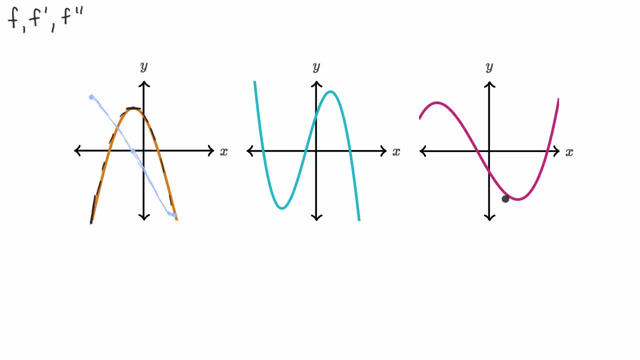 But what about this magenta graph? It does have, it does look like it has the right trend. In fact, it intersects the x-axis at the right place, right over there, and at least over this interval, it seems it's positive from here to here. 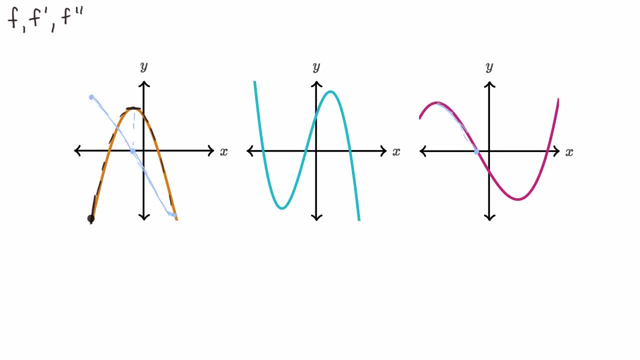 So it's positive. This graph is positive when the slope of the tangent line here is positive, and this graph is negative when the slope of the tangent line here is negative. Now, one thing that might be causing some unease: to immediately say that this last graph 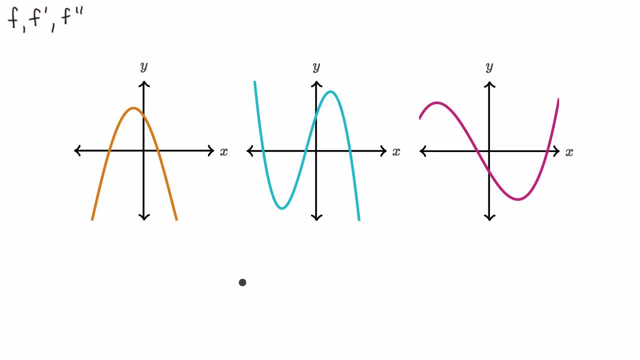 which one is f, which is the first derivative and which is the second. Like always, pause this video and see if you can work through it on your own before we do it together. All right, now, let's do this together, and the way I'm going to tackle it. 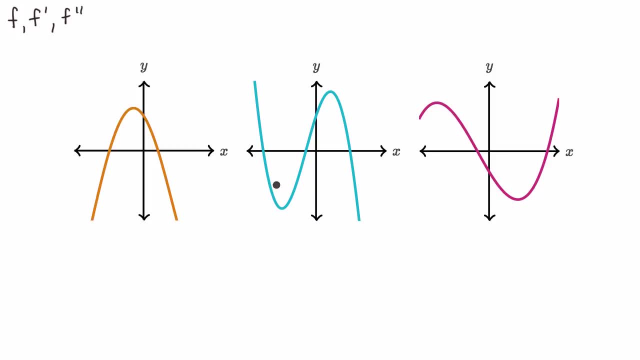 is. I'm gonna try to sketch what we can about the derivatives of each of these graphs or each of the functions represented by these graphs. So in this first graph here, in this orange color, we can see that the slope is quite positive here. 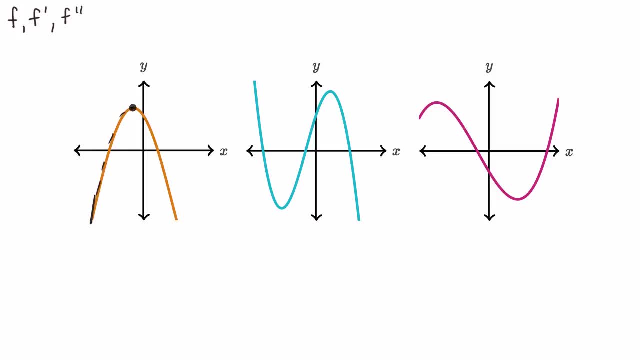 but then it becomes less and less and less positive, up until this point where the slope is going to be zero, and then it becomes more and more and more and more negative. So the derivative of this curve right over here, or the function represented by this curve, 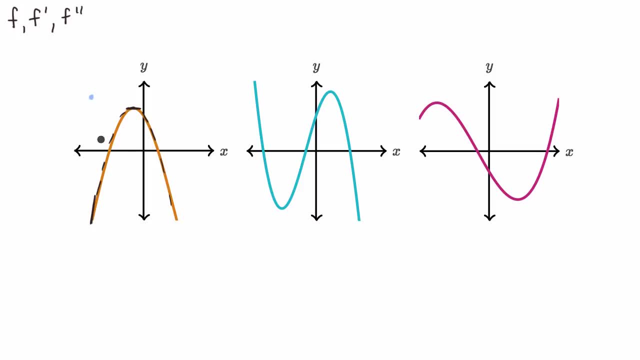 it's gonna start off reasonably positive. right over there At this point the derivative is gonna cross zero, because our derivative is zero there- slope of the tangent line and then it's gonna get more and more negative, or at least over the interval that we see. 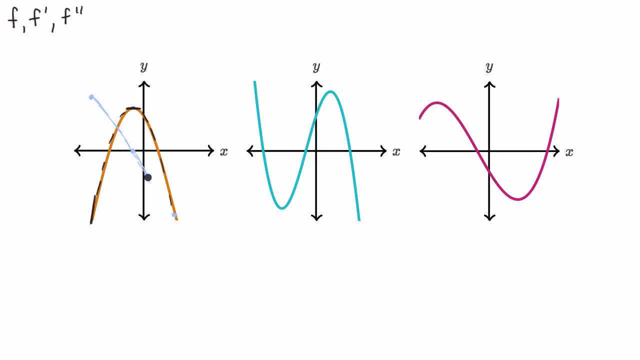 So it might look- I don't know- something like this. I don't know if it's a line or not, It might be some type of a curve, but it would definitely have a trend, something like that. Now we can immediately tell that this blue graph. 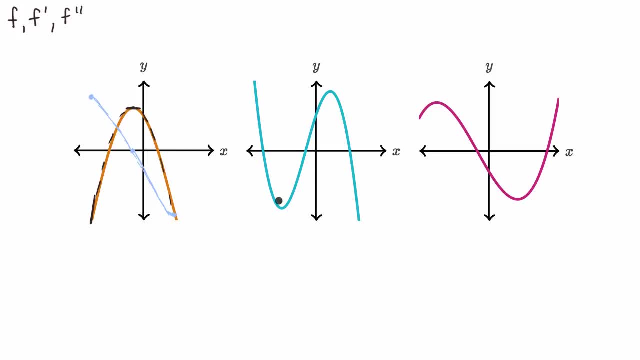 is not the derivative of this orange graph. Its trend is opposite. Over that interval it's going from being negative to positive as opposed to going from positive to negative. So we can rule out the blue graph as being the derivative of the orange graph. 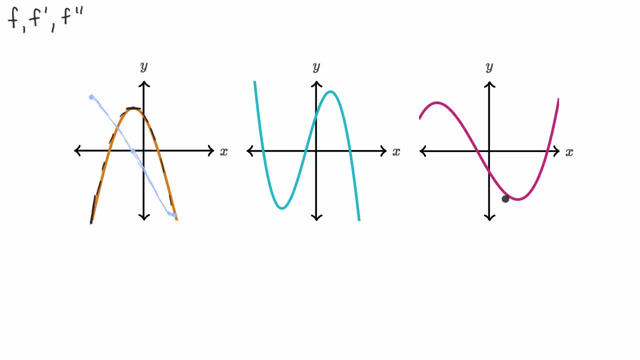 But what about this magenta graph? It does have, it does look like it has the right trend. In fact, it intersects the x-axis at the right place, right over there, and at least over this interval, it seems it's positive from here to here. 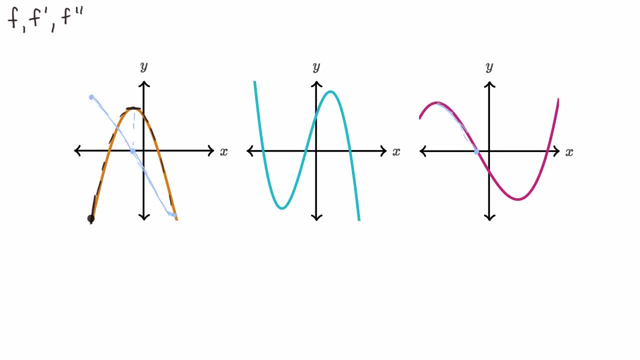 So it's positive. This graph is positive when the slope of the tangent line here is positive, and this graph is negative when the slope of the tangent line here is negative. Now, one thing that might be causing some unease: to immediately say that this last graph 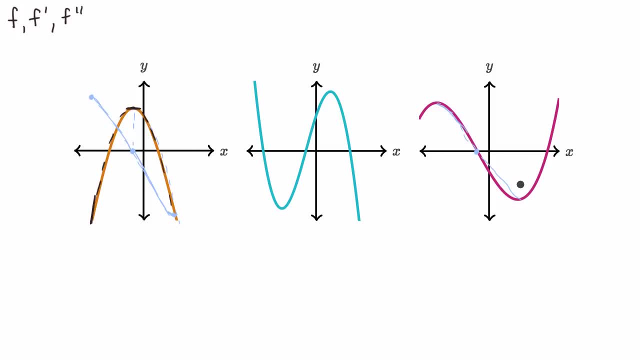 is the derivative of the first one is. we're not used to situations where the derivative has more extreme points, more minima and maxima, than the original function, But in this case it could just be because we don't see the entire original function. 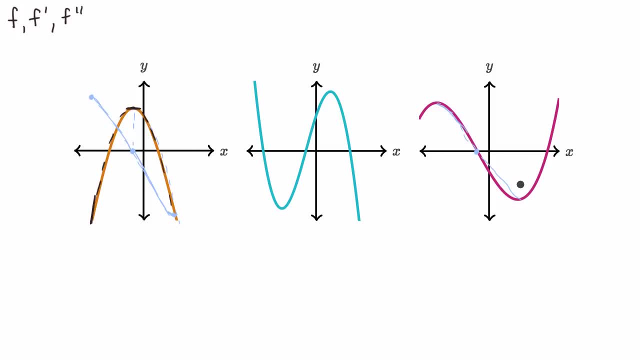 is the derivative of the first one is. we're not used to situations where the derivative has more extreme points, more minima and maxima, than the original function, But in this case it could just be because we don't see the entire original function. 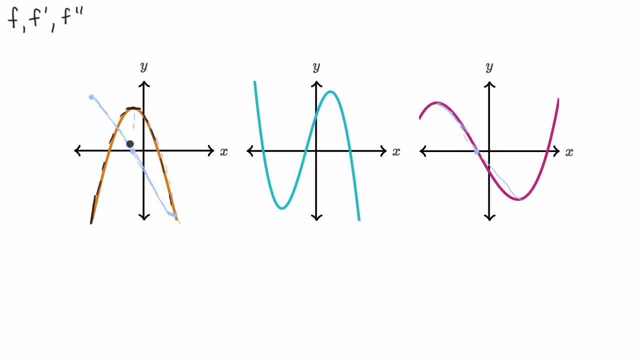 So, for example, if this last graph is indeed the derivative of this first graph, then what we see is our derivative is our graph. our derivative is negative right over here, but then right around here it starts becoming less negative. So if that point corresponds to roughly right over there, 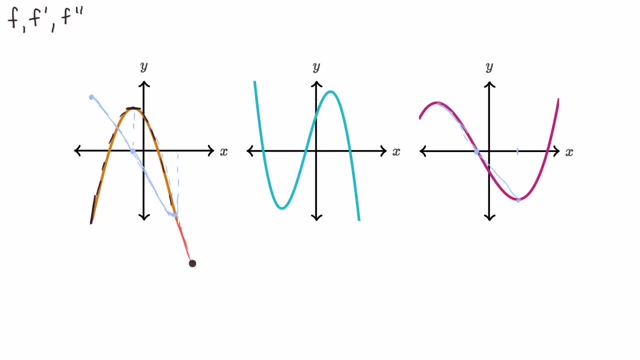 then over here, our slope will become less and less and less negative and then, at this point, our slope would become zero, which would be right around there. So, for example, our graph might look something like this: We just didn't see it. 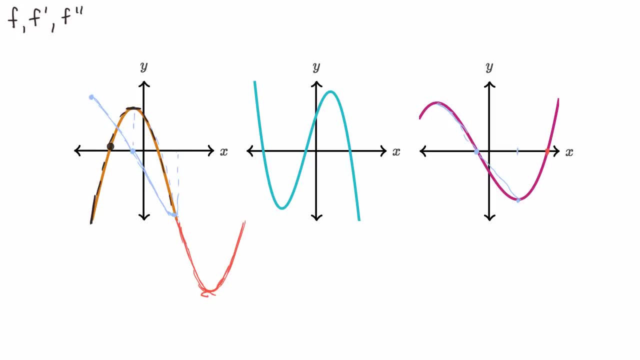 It fell off of the part of the graph that we actually showed, So I would actually say that this is a good candidate for being the third function, is a good candidate for being the derivative of the first function, So maybe we could say that this is f. 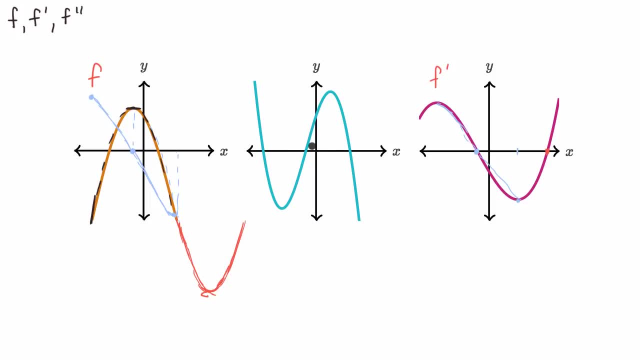 and that this is f prime. Now let's look at the second graph. What would its derivative look like? So, over here, our slope is quite negative, and it becomes less and less and less negative until we go right over here where our slope is zero. 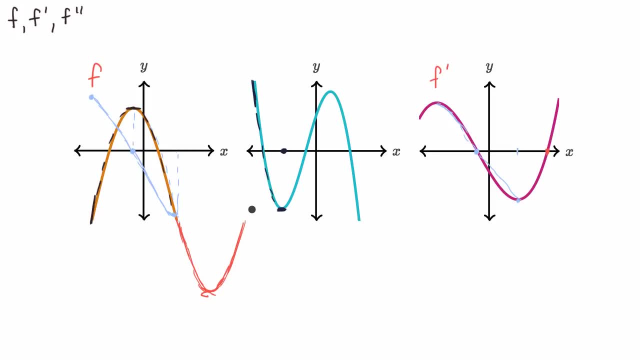 So our derivative would intersect the x-axis right over there. It would start out negative and it would become less and less and less negative and at this point it crosses the x-axis and then it becomes more and more positive. So we see here our derivative becomes. 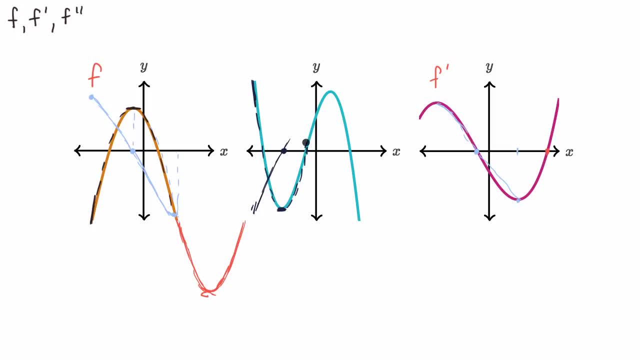 more and more positive, but then right around here it seems like it's getting less positive again. So it might look something. might look something like this: where over here it's becoming less positive again, less positive, less positive, less positive. 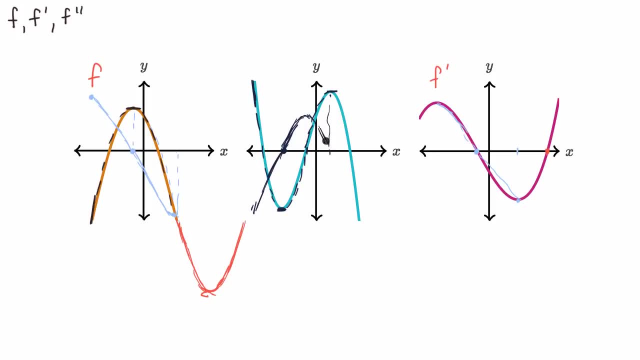 Right over here. our derivative would be zero, So our derivative would intersect the x-axis there and then it just looks like it is. the slope is getting more and more and more negative, So our derivative's gonna get more and more and more negative. 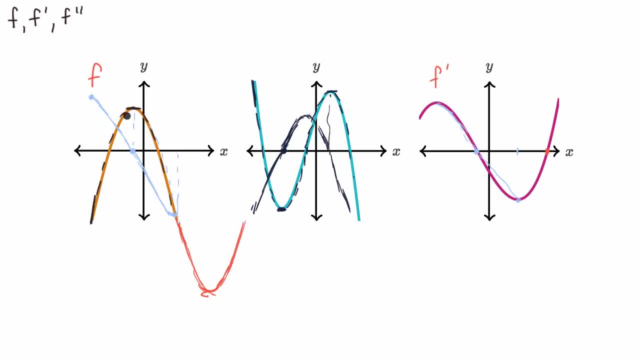 Well, what I very roughly just sketched out looks an awful lot like the brown graph right over here. So this brown graph does indeed look like the derivative of this blue graph. So what I would say is that this is actually f, and then this would be f prime. 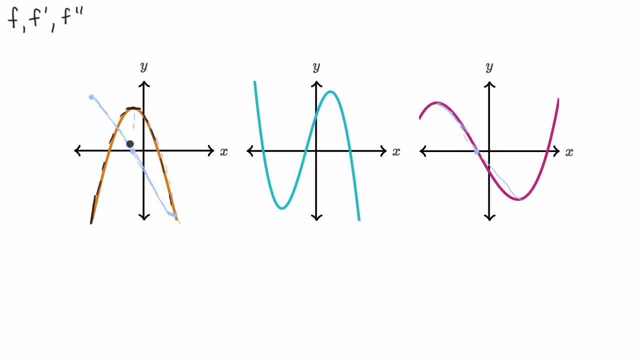 So, for example, if this last graph is indeed the derivative of this first graph, then what we see is our derivative is our graph. our derivative is negative right over here, but then right around here it starts becoming less negative. So if that point corresponds to roughly right over there, 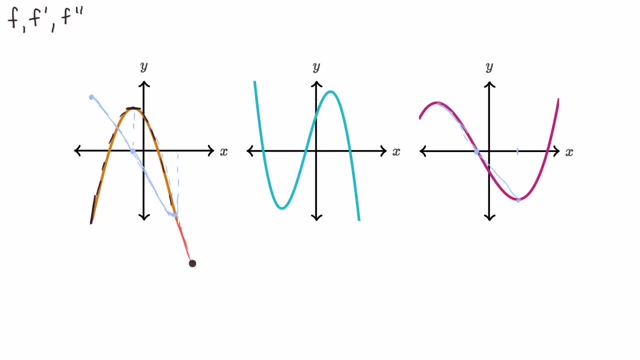 then over here, our slope will become less and less and less negative and then, at this point, our slope would become zero, which would be right around there. So, for example, our graph might look something like this: We just didn't see it. 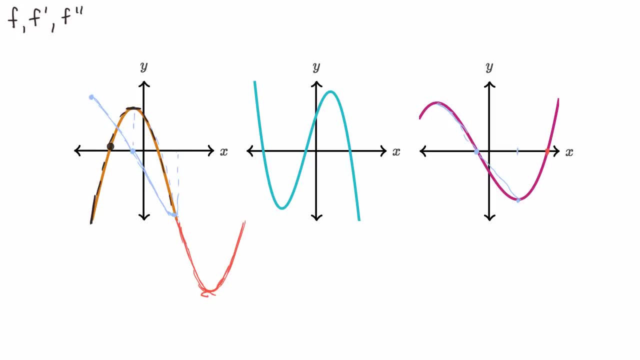 It fell off of the part of the graph that we actually showed, So I would actually say that this is a good candidate for being the third function, is a good candidate for being the derivative of the first function, So maybe we could say that this is F. 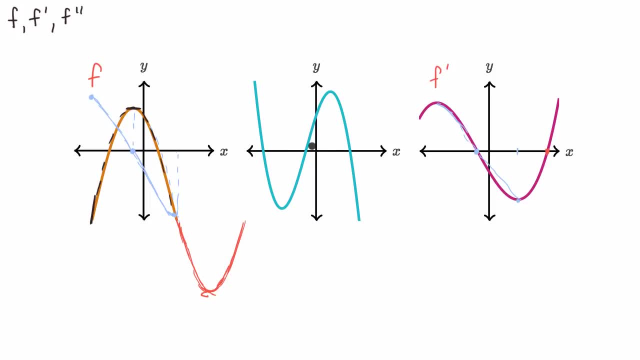 and that this is F prime. Now let's look at the second graph. What would its derivative look like? So, over here, our slope is quite negative, and it becomes less and less and less negative until we go right over here where our slope is zero. 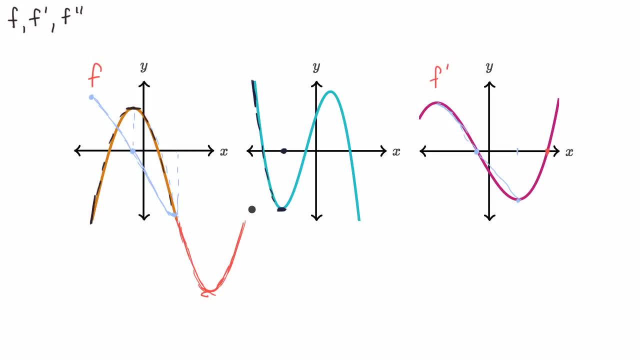 So our derivative would intersect the x-axis right over there. It would start out negative and it would become less and less and less negative and at this point it crosses the x-axis and then it becomes more and more positive. So we see here our derivative becomes. 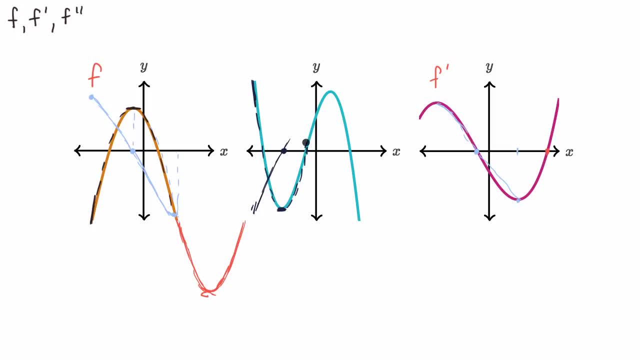 more and more positive, but then right around here it seems like it's getting less positive again. So it might look something. might look something like this: where over here it's becoming less positive again, less positive, less positive, less positive. 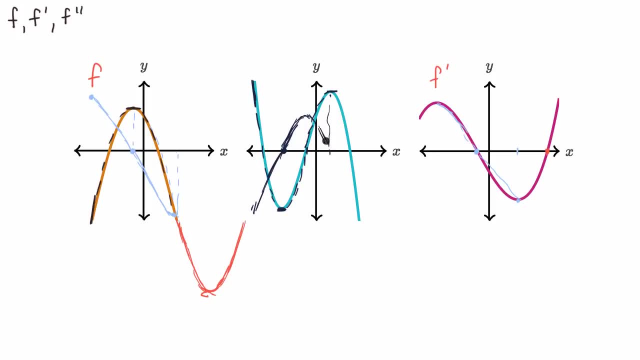 Right over here. our derivative would be zero, So our derivative would intersect the x-axis there and then it just looks like it is. the slope is getting more and more and more negative, So our derivative's gonna get more and more and more negative. 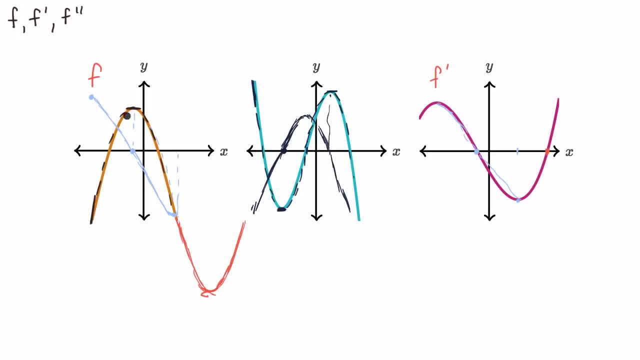 Well, what I very roughly just sketched out looks an awful lot like the brown graph right over here. So this brown graph does indeed look like the derivative of this blue graph. So what I would say is that this is actually F, and then this would be F prime. 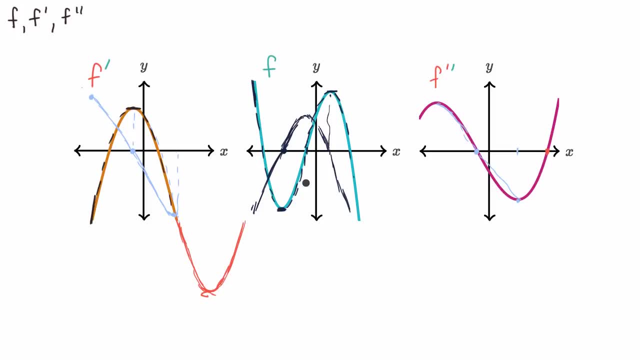 and then if this is F prime, the derivative of that is going to be F prime prime. So that looks good. I would actually go with this And if you wanted, just for safe measure, you could try to sketch out what the derivative of this graph would be.